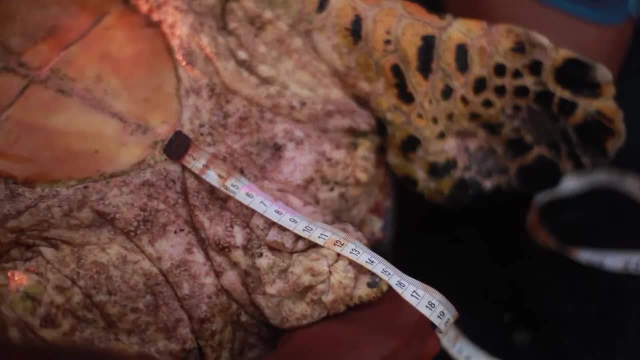 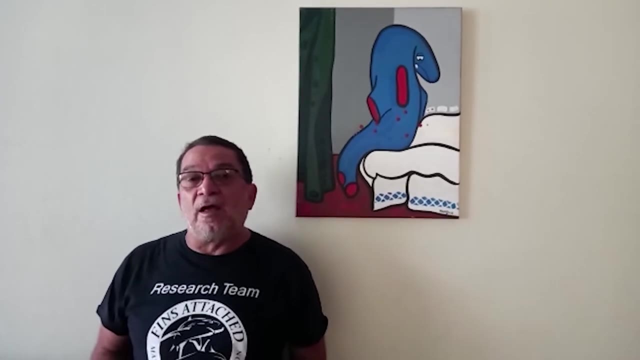 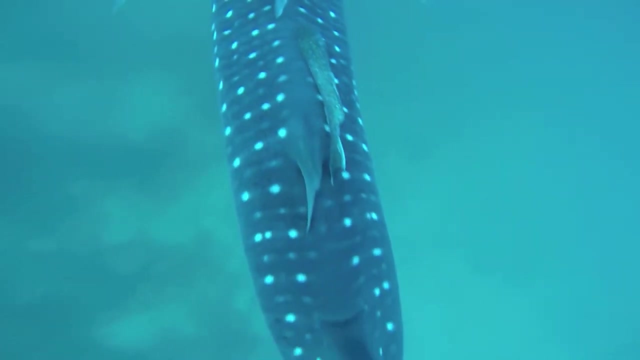 International Union for the Conservation of Nature, precisely because of their overfishing. Overfishing is one of the main problems that we have to face right now. we're trying to solve- and there are two basic solutions for this: Finding sustainable livelihoods for people who live in coastal communities, and the 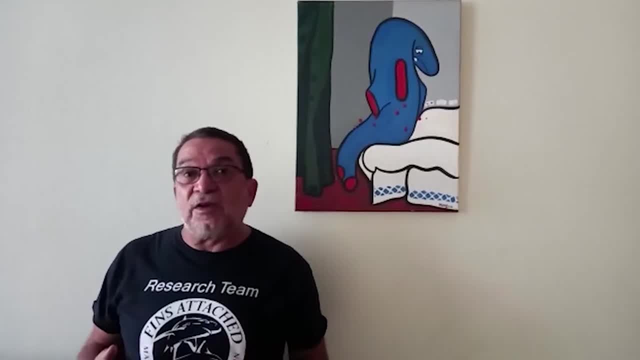 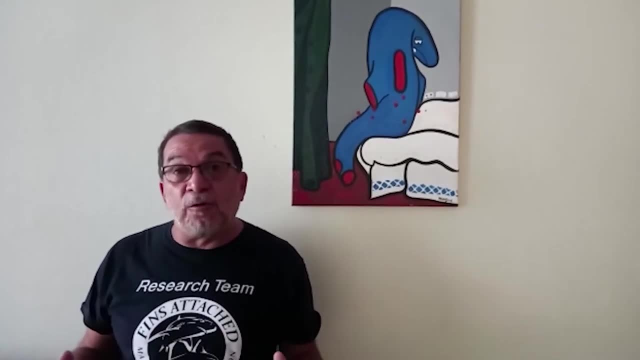 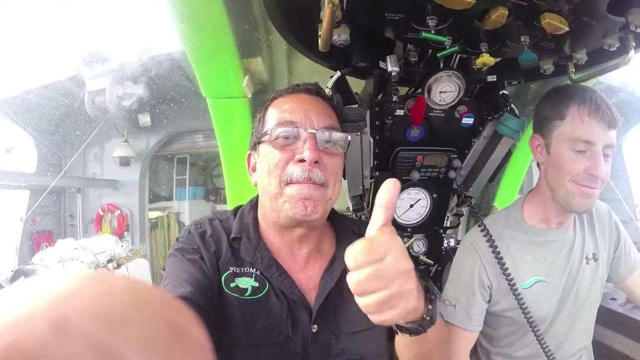 second one is: we definitely need high seas marine protected areas where no fishing is allowed, and we already know that the bigger these marine protected areas are, the better they are for marine conservation and the better they are for commercial fisheries. Throughout my career, I have worked on influencing 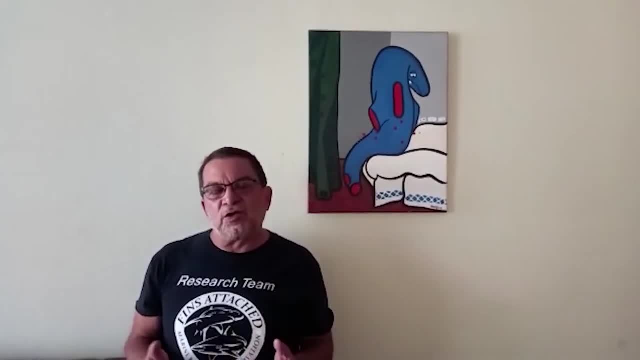 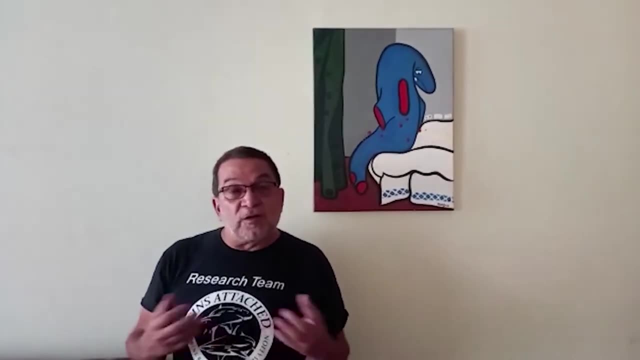 policy for the better, for the improvement of marine conservation. I have worked in Costa Rican courts, I've worked in international courts, I've worked in conventions. we've been very successful in many fields. we've had a lot of impact and there's one thing I've learned and I would like to share with. 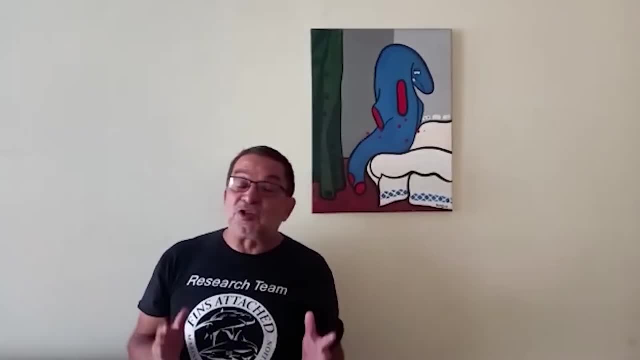 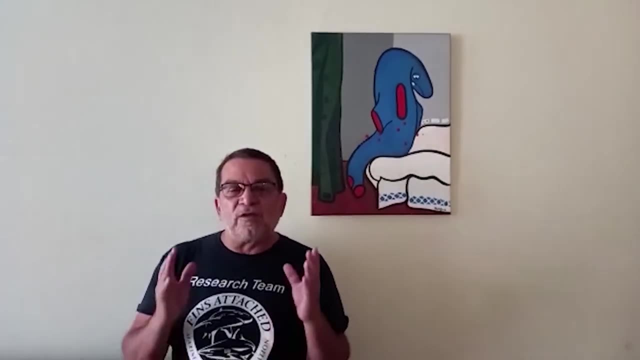 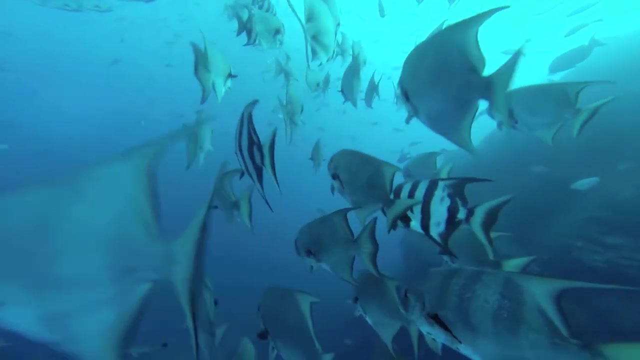 everyone who's trying to do marine conservation policy, especially nowadays, that it's a good thing. It's so critical and so important. We must work with our environment authorities and we must work with our domestic conservation of wildlife laws and conservation of biodiversity laws. but as soon as we start working in these, 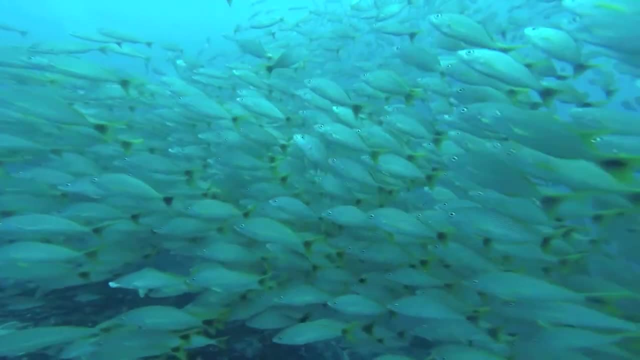 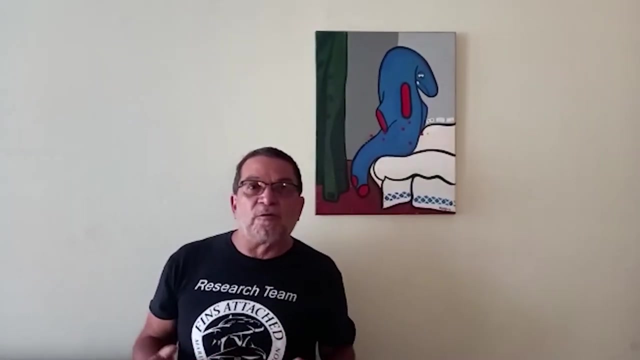 fishery conventions in which are with our fishery authorities, we start seeing this unwillingness to abide by the best scientific evidence possible and of course this does not work for the conservation of the species we're working so hard to protect. So let's do everything we can to protect our 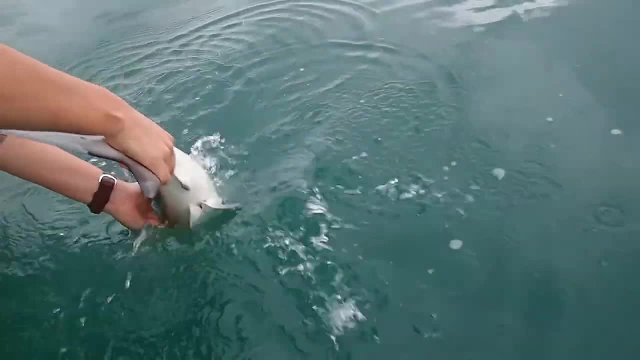 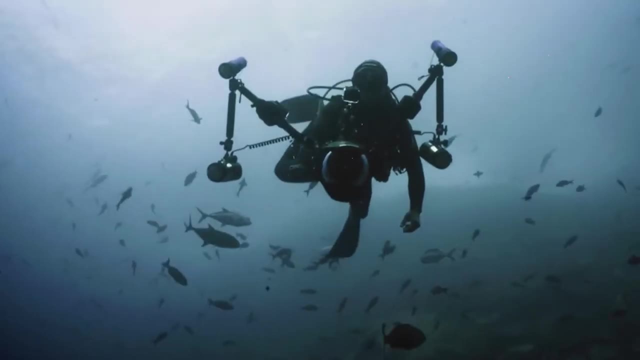 environment, to empower our authorities of environment so that we can move forward and save these animals. What makes this project unique is, first of all, we're scientists. We're concerned about generating the best science, working with the best scientists, so we can provide the authorities with the 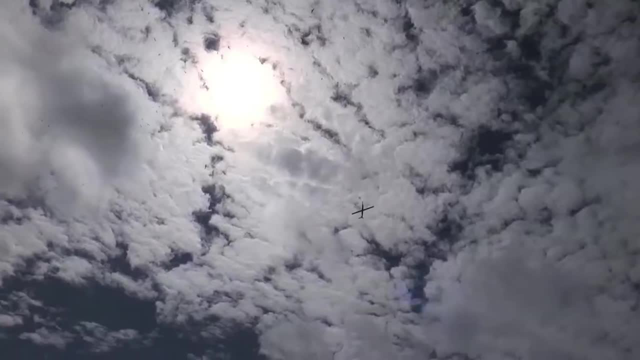 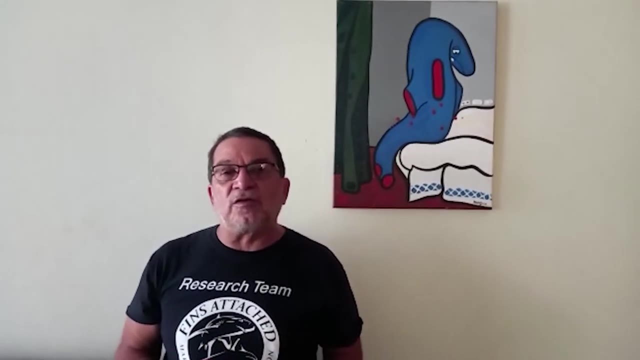 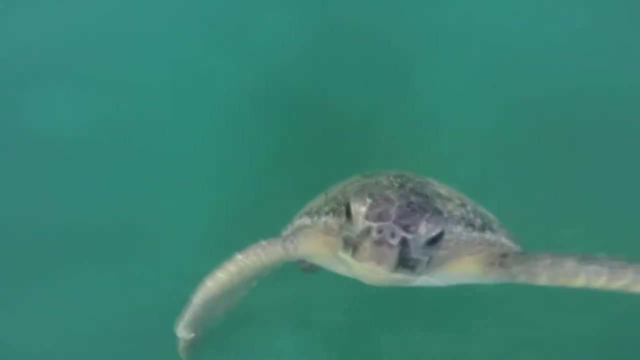 best advice on how to improve marine conservation policy. On the other hand, we're aware of the law. We know our laws very well. we know conservation law, biodiversity laws in Costa Rica. We handle them all pretty well And we actually handle international law pretty well as well. And what?